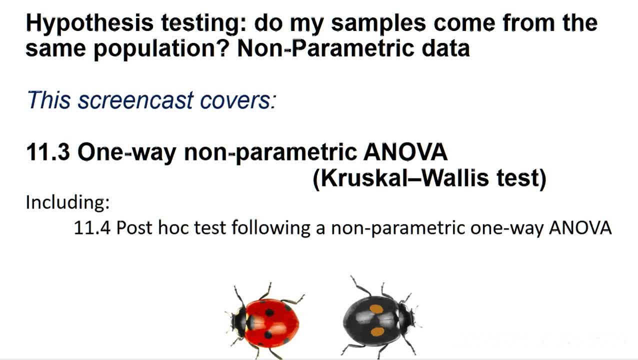 an extent from each other that they can be considered to come from different populations. This test is a non-parametric test. If you do not understand what this means, then please see my screencast. Is My Data Normally Distributed In the example we are using here, eight quadrats. 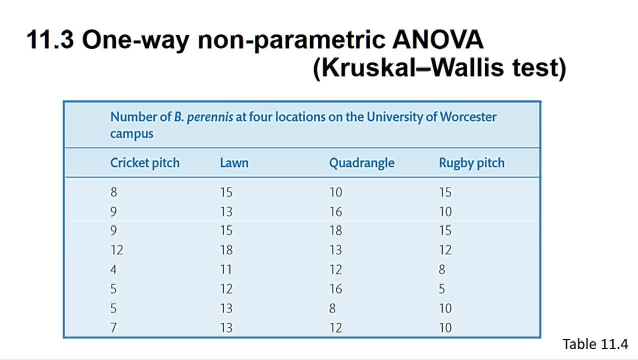 were sampled for the number of daisy plants growing in the Biosciences screencast. The data is being sampled in four distinct grassed areas with different uses at the University of Worcester. These areas were the cricket pitch, the lawn, the quadrangle and the rugby. 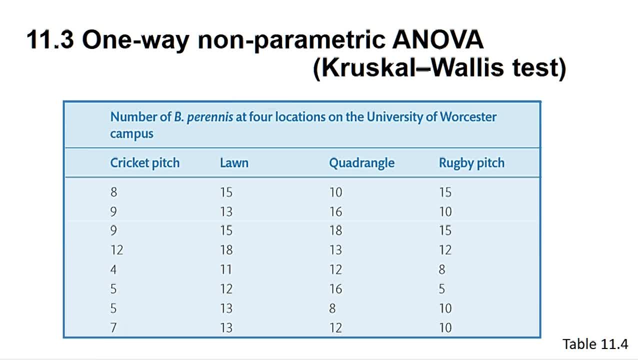 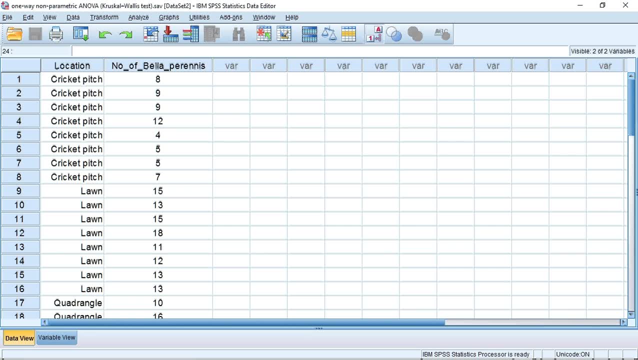 pitch. The data can be found in Table 11.4.. I have already entered the data into SPSS. Please see the web walkthrough for more details on how to set the variables up. Please note that the web walkthrough details a simpler method of doing this test, but the advantage of the following method is that it will also do the post hoc test for the non-parametric one-way ANOVA. Please note that the web walkthrough details a simpler method of doing this test, but the advantage of the non-parametric one-way ANOVA is that it will also do the post hoc test. 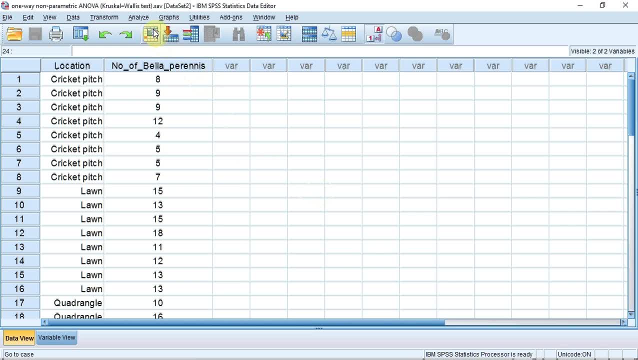 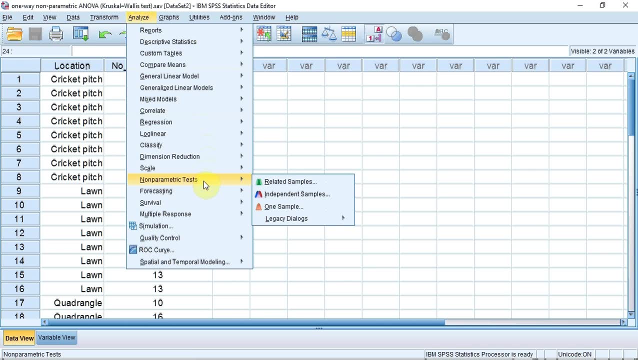 for the non-parametric one-way ANOVA. To do the non-parametric one-way ANOVA, we go up to Analyse and click. A submenu drops down. It is a non-parametric test, so we go down to Non-parametric tests. It has four independent samples, so we go to the submenu. 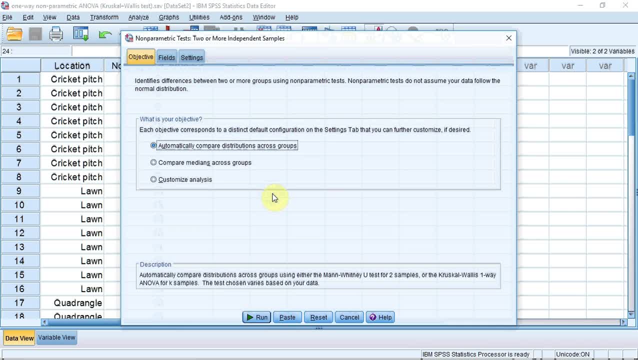 and click Independent samples and the following window opens. At this point, you could click Run and SPSS will make an educated guess at the test that you need to analyse your data. However, we know the test we want to use, so I am going. 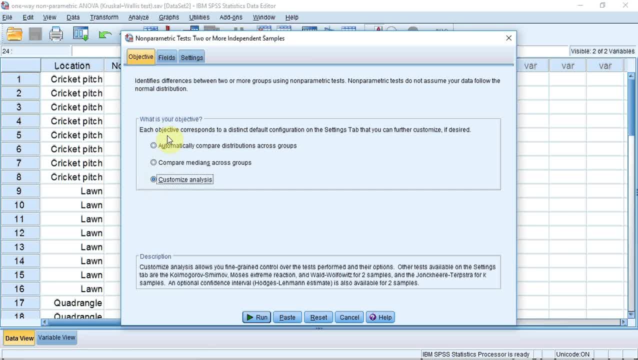 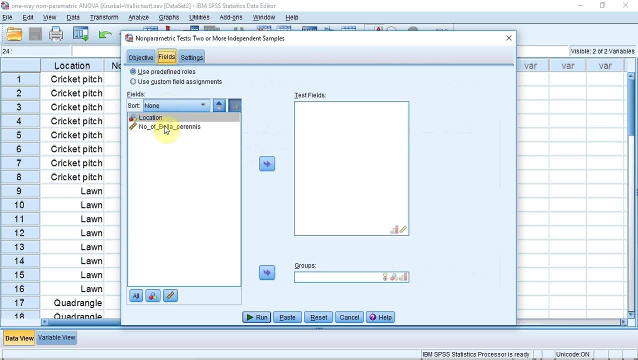 to click the Customise test. I am now going to track up to the Fields tab and tell SPSS which variables I want it to analyse. The test fields variable is the number of daisy plants, Bella perennis. I am going to select that and enter it into the test field box using the selection arrow. We are 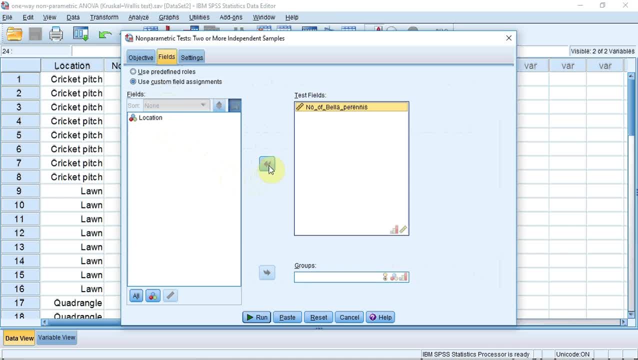 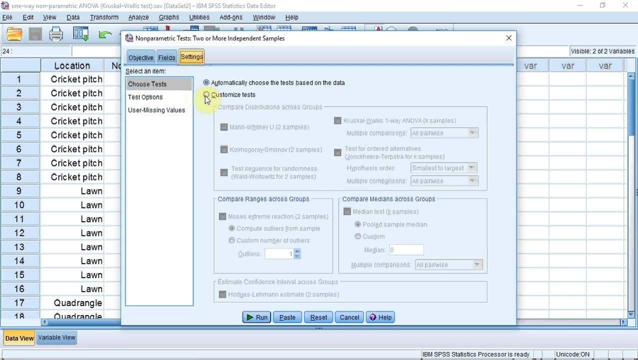 going to divide that data up into four groups and the information for that is stored in the Location variable, which I am going to select, and I am going to enter it into the Groups box. I am now going to go back up to Settings to tell it which test I want to use. I click the Settings tab and I click the Customise. 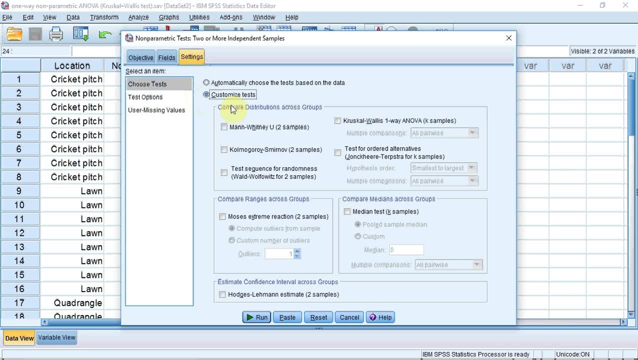 test radio button. You can see it has several tests, including the Kruskal-Wallis one-way ANOVA. I am going to tick the box. It also allows me to select how I want to compare the data afterwards using the post hoc test. I am going to leave it as All-Pairwise. I